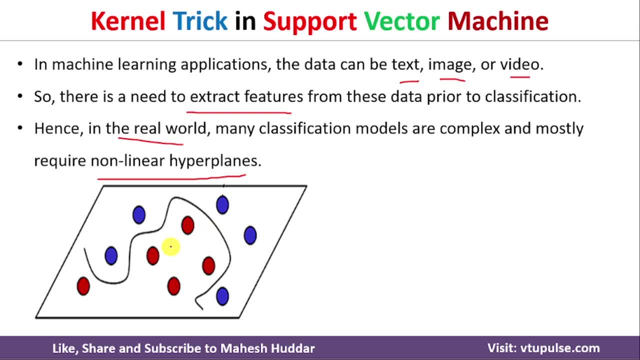 it is very complex To avoid this particular thing. what we need to do is we need to convert this particular data, That is, nonlinear data, into linear data. It may be something like this: It is a 2D data, But in. 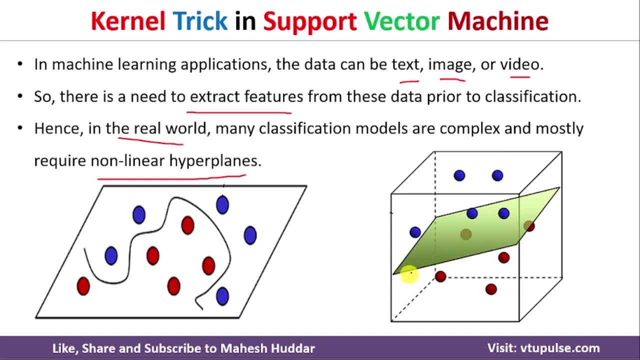 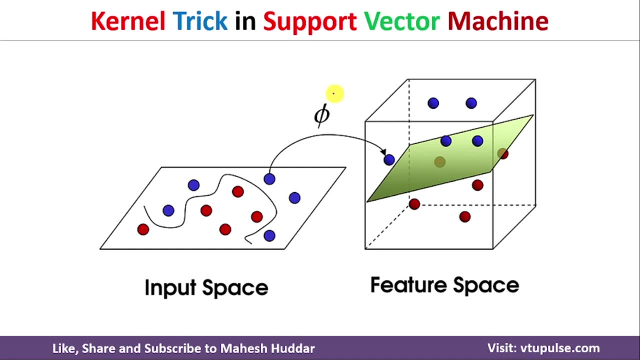 this case. you can see here, it is a 3D data And we will be able to separate this particular data with the help of a plane over here. So this is what is called as converting the data from one space into another space over here. So what we need to do, we need to apply a mapping function. 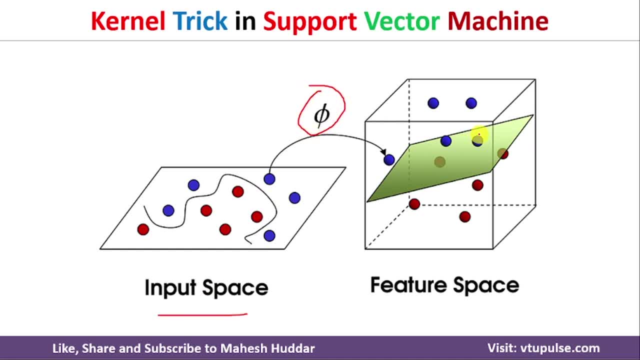 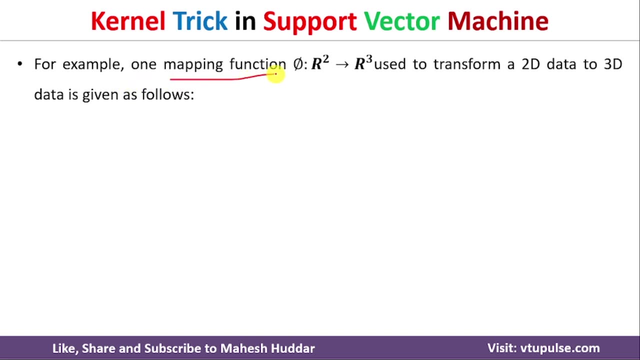 on the input space and then convert this particular nonlinear data into a linear data That will be called as a feature space over here. And what is that particular mapping function That depends on the given data set over here? Now we will take an example to understand this particular mapping. 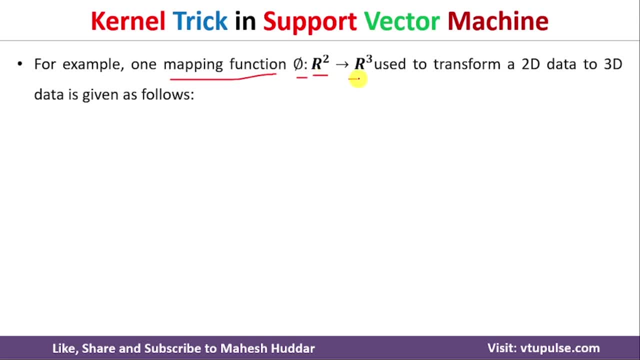 function. Let us say that phi is a mapping function from R square to R3.. That is nothing, but we want to transform the data from 2D data to a 3D data. So the mapping function for x- y, that is a 2D data, looks something like this: Phi of x- y is equal to. 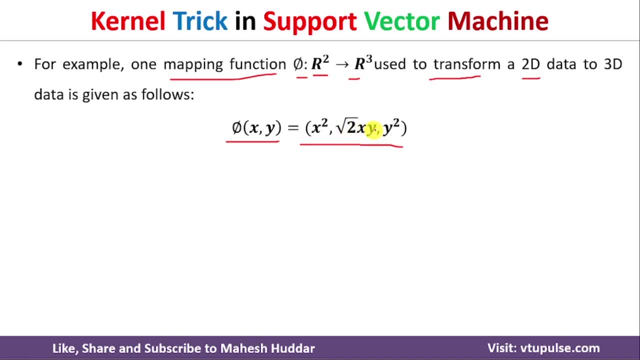 x square comma, square root of 2, multiplied by x, y comma, y square over. here. Let us say that a point 2, 3 is a data point in a 2D space And if we apply this particular mapping function on this particular thing, we will get a data into 3D space. So in this case the value of x is 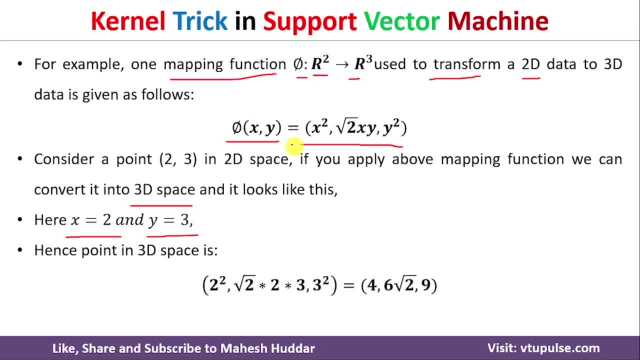 equal to 2 and y is equal to 3.. And phi of 2, 3 is equal to 2, square comma, square root of 2, multiplied by x, multiplied by 2.. So this is the mapping function And if we apply this particular, 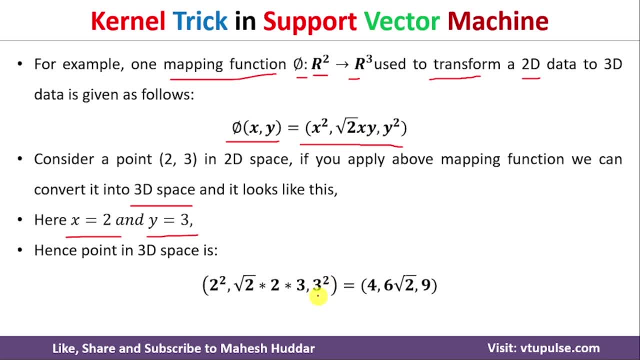 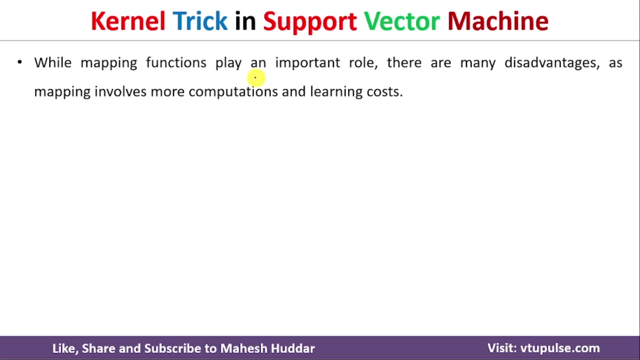 mapping function. we will get a data into 3D space, So the mapping function plays a very important role when you want to transform a data set from one space to another space, that is, input space to another space. So this is the mapping function. 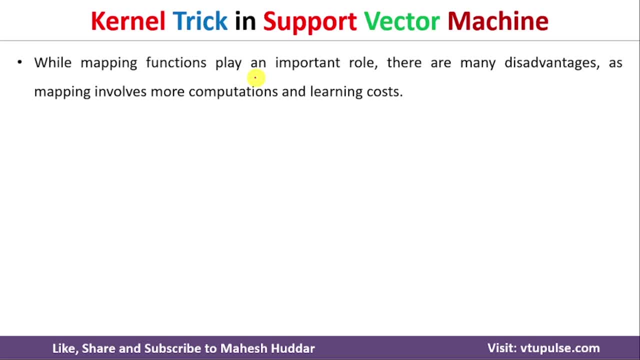 But these mapping functions have a lot of disadvantages. Some of them are computational cost as well as the learning cost. Along with this particular thing, the very important disadvantage is there is no generalized thumb rule available for what transformation should be applied for the given data set. For example, there is a data set given to us that is D1 and 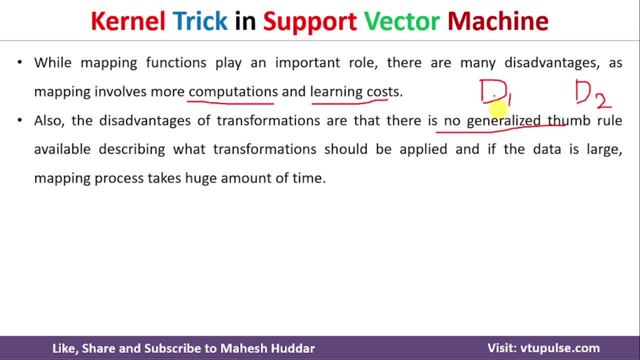 there is another data set given to us that is D2. You cannot say that, whatever the transformation you have applied on that data set, you cannot say that you have applied on that data set. But you can say that you can apply on D1,, you can apply on D2 also. There may be a possibility. 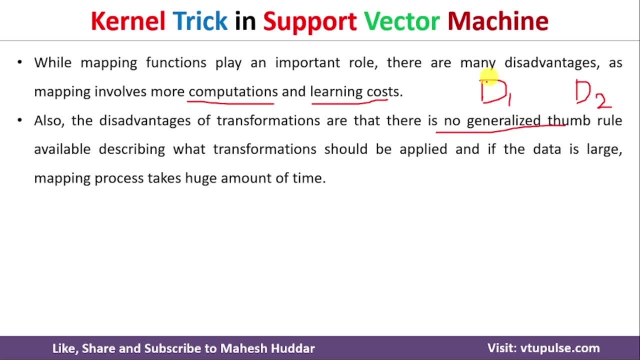 that we can apply, but it is not a generalized rule that what you apply over here, it will work on this particular D2 also. So for each and every data set we will get different mapping functions over here. So that is the reason you can say that there is no generalized. 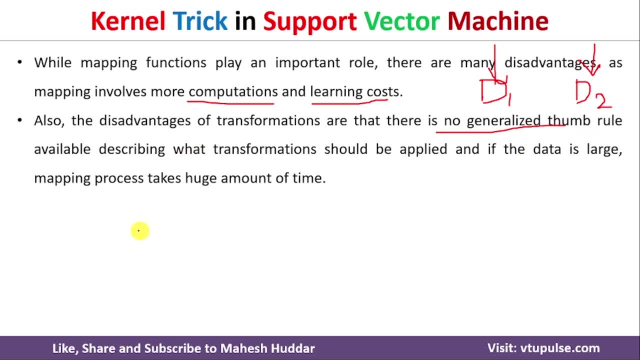 thumb rule for describing the transformations over here. And when the data set become too large, it will take a lot of time to transform the data from one space into another space over here. At the same time, it will take a lot of computational cost, as said earlier, as well as it will take 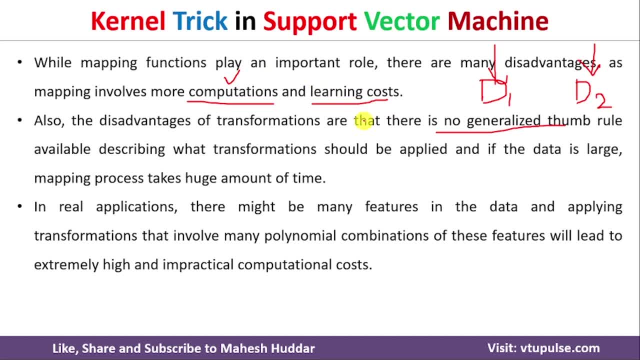 a lot of time to convert that particular data from one space into another space over here. In this particular case, we need to use something called as the kernels. They will come handy in this particular case. So kernels are used to compute the value without transforming. 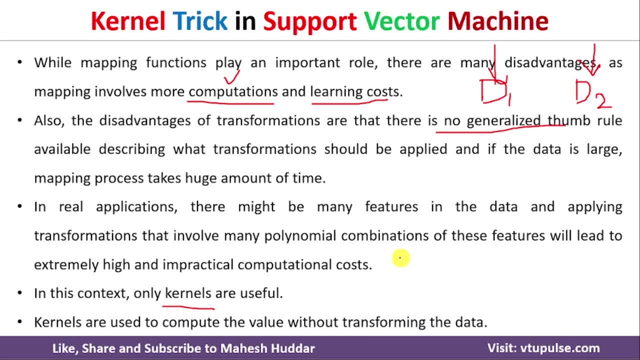 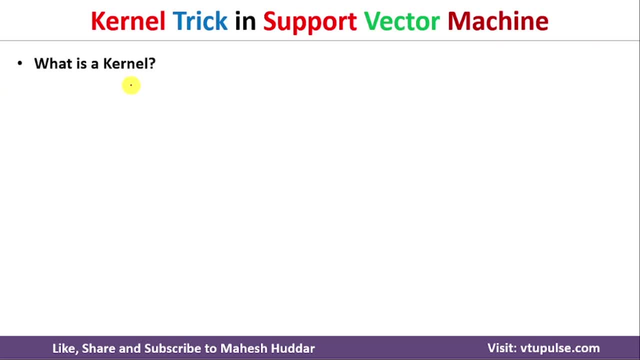 the data. We don't transform the data over here. We will use the dot product to represent the low-dimensional data data into high dimensional data over here. so what is kernel? that's the next question comes in front of us. kernels are the set of functions used to transform a data from low dimensional into high. 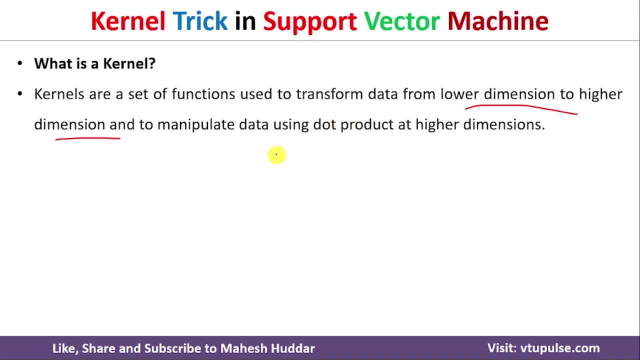 dimension. over here they manipulate the data using the dot product at the high dimensional rather than converting a data from one space into another space. the working principle of kernel is shown over here. given a low dimension data, once you apply the kernels on the top of it, you will. 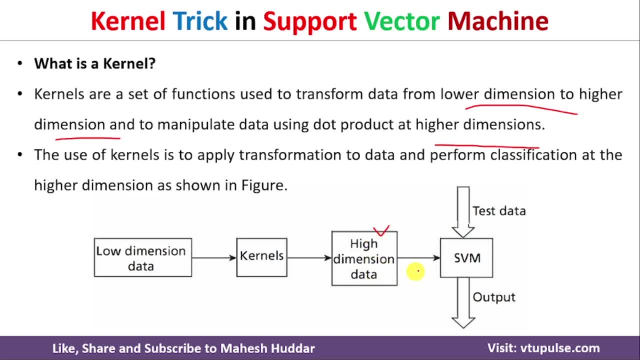 get a high dimensional data on the top of this particular high dimensional data. we need to perform the classification over here again. as said earlier, we are not going to convert this particular low dimension data into high dimensional. we are going to map the low dimensional data into high dimensional with the help of something called as a dot product over. 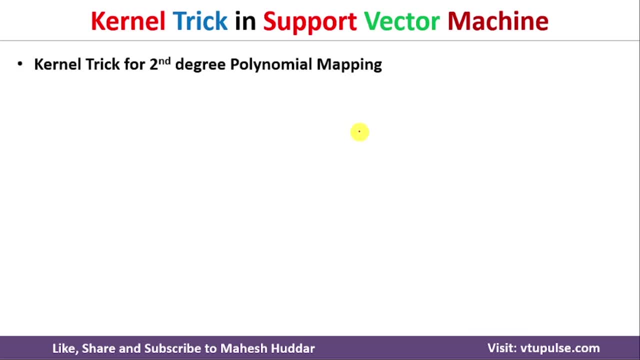 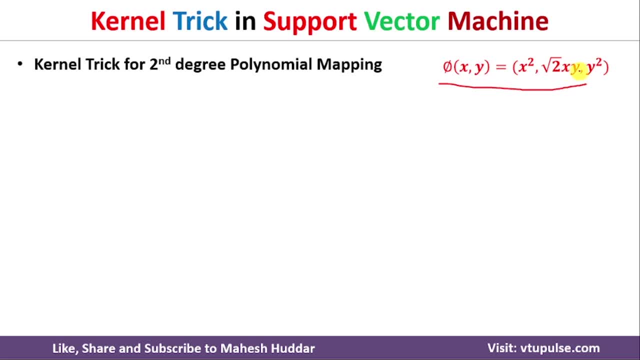 x square comma square root of 2 x, y comma y square. this is the mapping function, so whenever we have been given a data x comma y, we need to apply this particular polynomial so that we will get the data in the 3d space. but it has to be done for each and every data point. that will be costly, so that is. 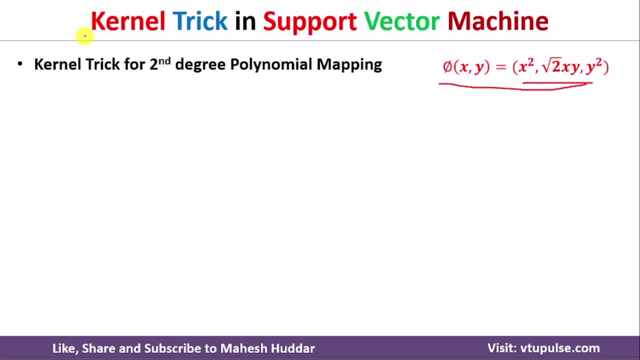 the reason. what we need to do over here is we need to use something called as the kernel trick over here. let us say that a and b are the two data points. the first data point, a, contains a1 and a2 as the feature values. b contains b1 and b2 as the feature values over here. so phi of a transpose that. 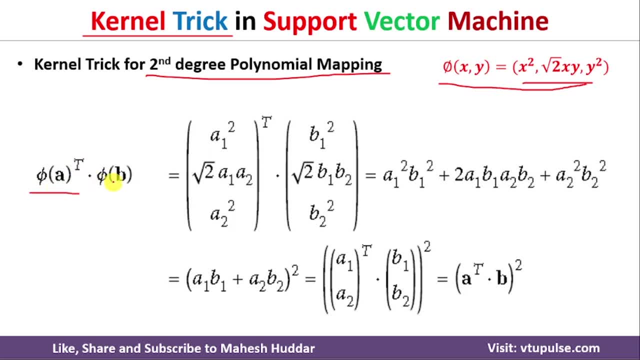 is the phi of a is the mapping function and its transpose dot. phi of b is equivalent to. so phi of a is nothing but what? a1 square, because it contains a1 and a2 as the feature values here. so a1 square, comma, square root of 2, a1, a2 comma, a2 square. so that is what i have written here, its transpose. 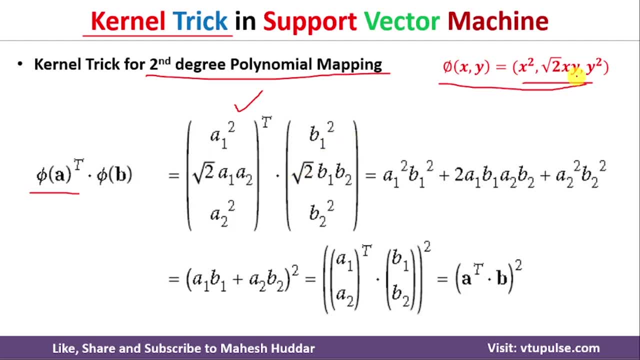 dot product with b1, square, square root of 2, b1, b2, b2 comma, b2, square over here. so once you multiply these two things, that is this matrix. with this matrix you will get. first you need to convert it into transpose here. so a1 square multiplied by 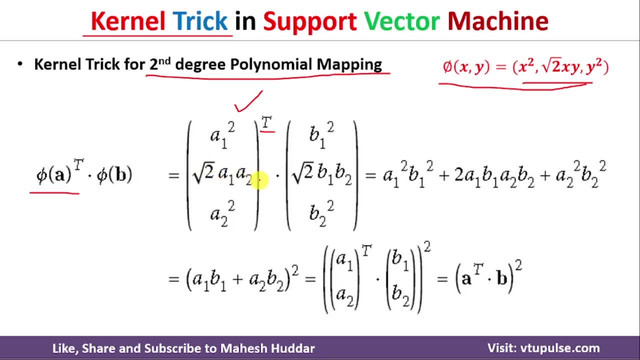 b1 square plus square root of 2, a1, a2, multiplied by square root of 2, b1, b2, multiple plus a2 square, b2, square over here. now, if we simplify this part, i think you will get a1, b1 plus a2- b2 bracket. 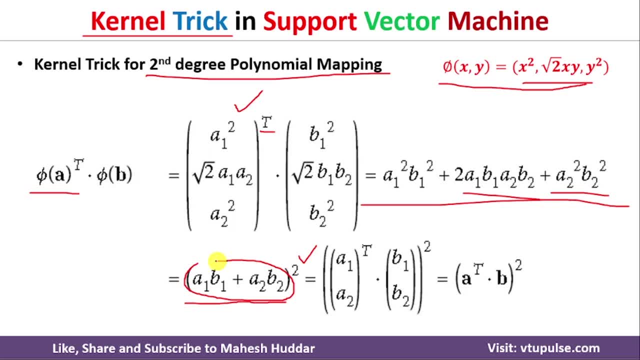 square over here. now how to get this part. i think here we come across the kernel trick here. so to get this particular a1, b1 plus a2, b2, we can write it something like this: a1, a2 as the feature values of a its transpose dot product with b1, b2, square over here. so if we take the 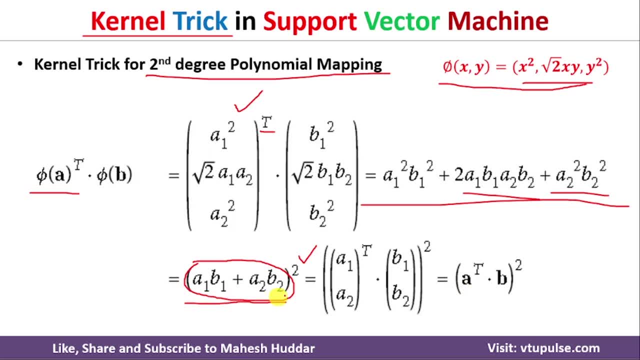 transpose and then multiply it to this one, you will get the a1, b1 plus a2, b2, square. so that is nothing but this equation. this is nothing, but you can say that the transformed point with the help of mapping function over here if you apply the second degree polynomial mapping each of those particular data. 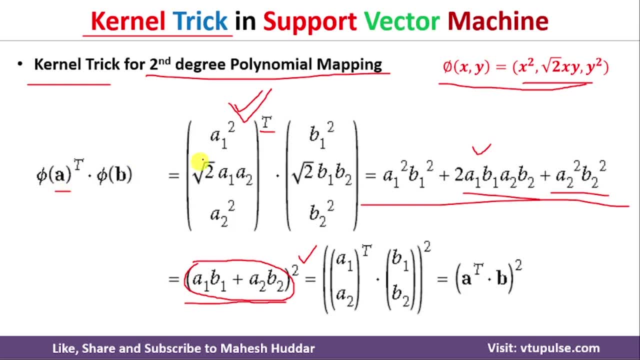 points must be converted into something called as the mapping values. so this is how actually we need to do it. this is the first one, this is second one, the same thing should be done for the third one, and so on, but rather than doing it for each and every data point in the kernel trick, what we 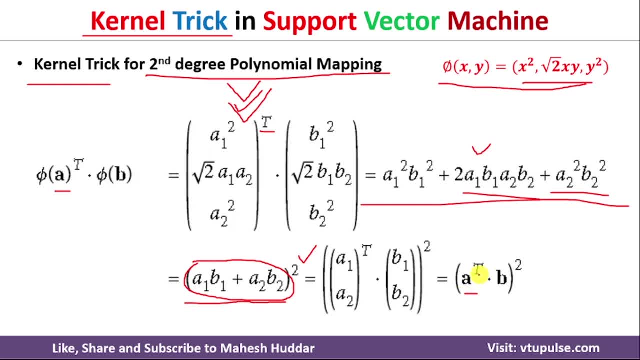 can do here is we can take that particular data point, its transpose dot product, with the second data point, so we are not actually converting it. what we are doing here is we are actually are taking the dot product between those two data points and then we are going to apply the 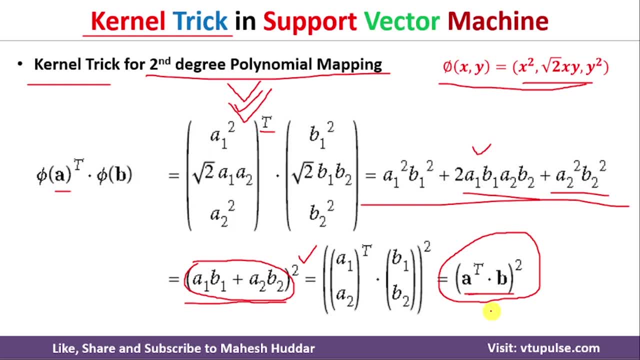 classification algorithm over here. so if you do this part, i think it will save a lot of computational costs as well as it will save a lot of learning time over here. if you do it without kernel trick, it will take a lot of time because each and every data point should be. 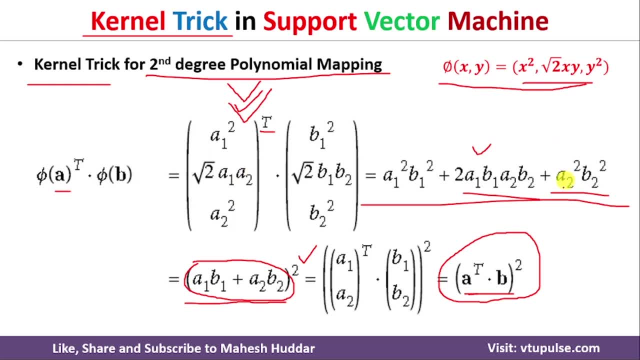 converted into a 3d space and then we need to apply the classification algorithm. but here what we are doing, we are taking the dot product between the data points and then we are going to apply something called as the classification algorithms. over here now we will try to discuss what are the. 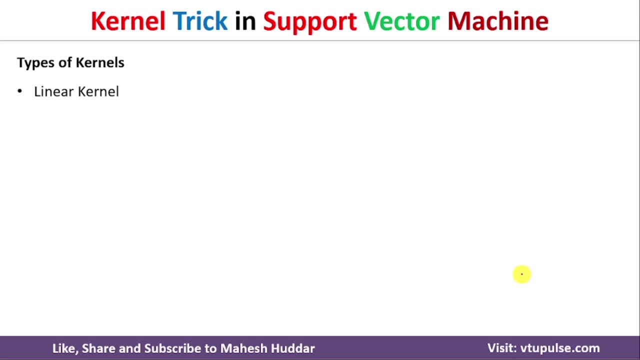 different kernel types are available in svm. so the first one is called as linear kernel. we have something called as polynomial kernel, exponential kernel, homogeneous kernel, inhomogeneous kernel, gaussian kernel, hyperbolic or the sigmoid kernel, radial basis function kernel and so on. so in this video i have discussed what is a mapping function in support function. 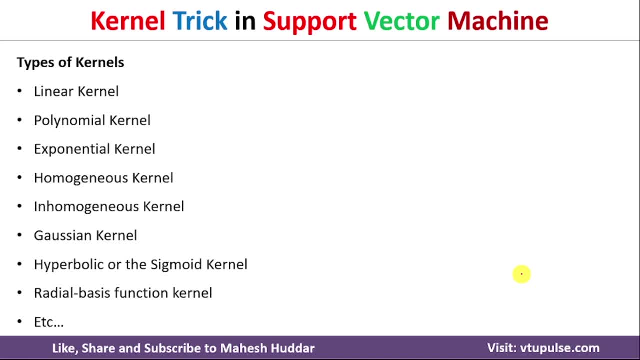 vector machine. what is kernel as well as kernel trick, and what are the different types of kernels available in support vector machine? in the next video i will discuss each of these particular kernel types in detail and later we will take a numerical example to understand the kernel trick. 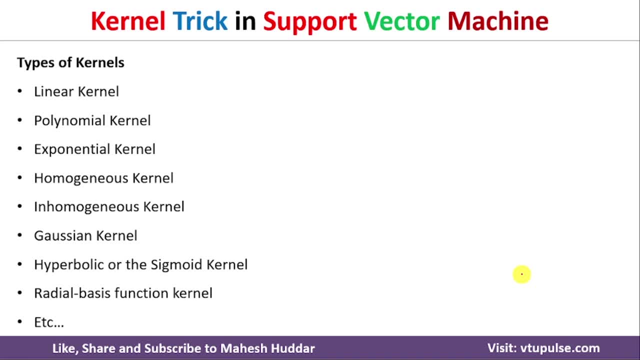 i hope the concept is clear. if you like the video, do like and share with your friends. press the subscribe button for more videos. press the bell icon for regular updates. thank you for watching.